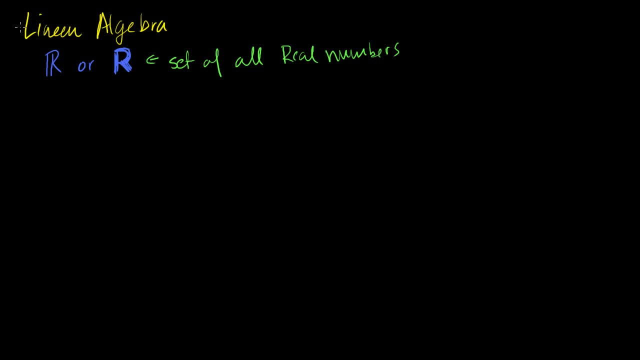 defining the set of all real numbers. But the simple thing for me is all numbers except complex ones. So this is the same thing as everything, Everything but complex, Complex numbers. So pi is a real number. e is a real number. Square root of 2 is a real number. 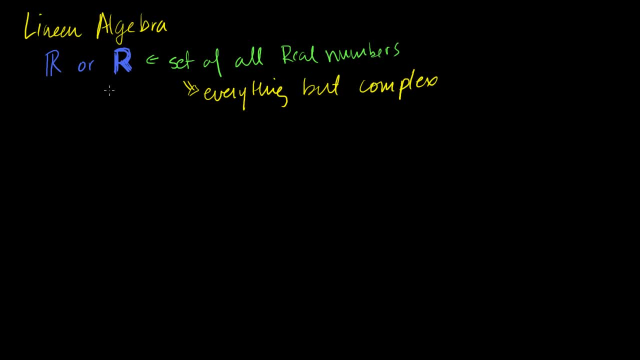 3 is a real number, Minus 3 is a real number, Minus pi is a real number. But 1 plus 2i not a real number, Not in the set of reals. That's a complex number. 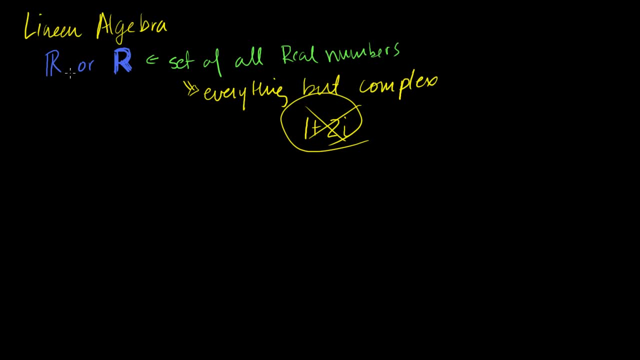 So everything but complex, So pretty much all regular numbers that you ever dealt with Before you learned what i was. That's the set of real numbers. Now the next thing you'll see when you start discussing linear algebra is someone will write. they won't just write. 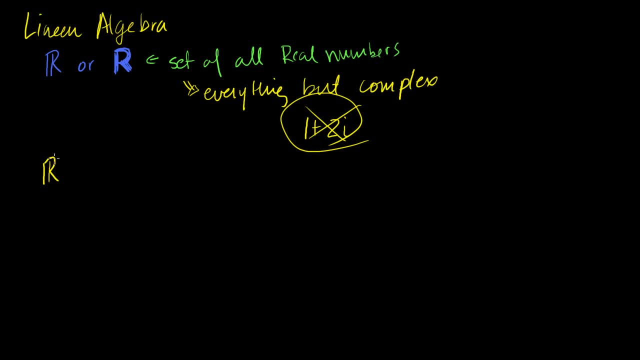 the set of all real numbers, They'll write r. I'll just write it generally. They'll write rn And you're like gee, what is that? Somehow are they somehow taking the exponent of all of the real numbers And actually, on some level, that is what they're doing. 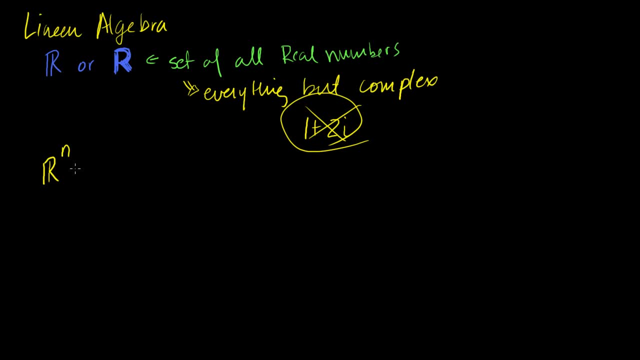 But what they're saying here is: you're taking the set of all ordered sets of real numbers. So what do I mean by that? So let me do an example where I don't just have rn. So r2 is the set of all lists of real numbers. 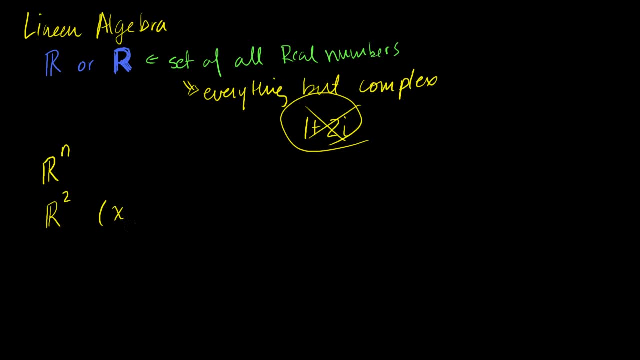 And let me make one of the lists. So let's say it has one number and then it has another number. Let me write it this way So I can write it in a set of notations. It's the set of all We could call these. 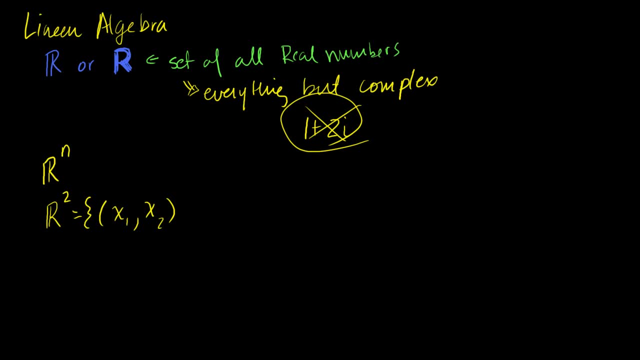 Tuples. Sometimes it's called a two-tuple, Which just means just a list of two numbers. That's all it means. It just means a list of two numbers. So r2 is the list of all ordered two tuples. So all ordered lists of two numbers. 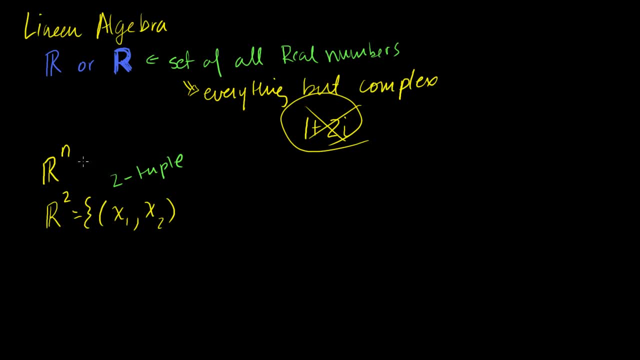 Let me actually write down the word ordered, because that's important. So: ordered list of two tuples. So, for example, this would be well, let me write it this way. This would be a different. when I say ordered, I'm saying: 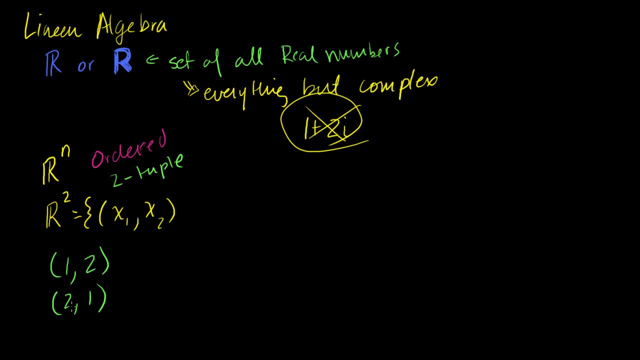 that this is fundamentally different than that, That these aren't the same two-tuple. Each of these is a two-tuple, But r2 is the set of all two tuples, such that that line there just means such that, or maybe for which, such that each. 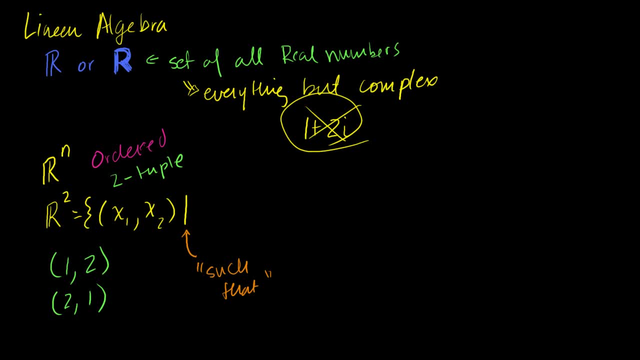 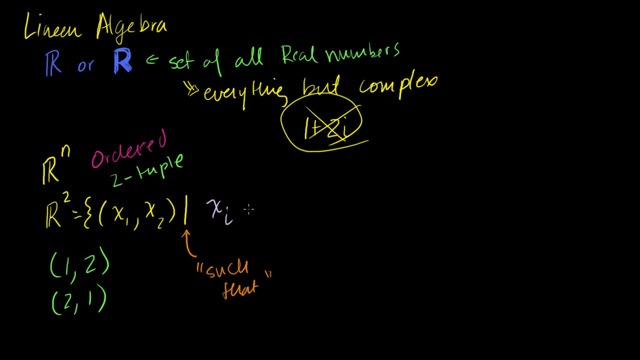 Just so you get used to it, Such that xi is a member of the reals. So member of, That's what this little character means, So that each xi is a member of the reals. What do you mean xi? Well, xi just means any of these x's. 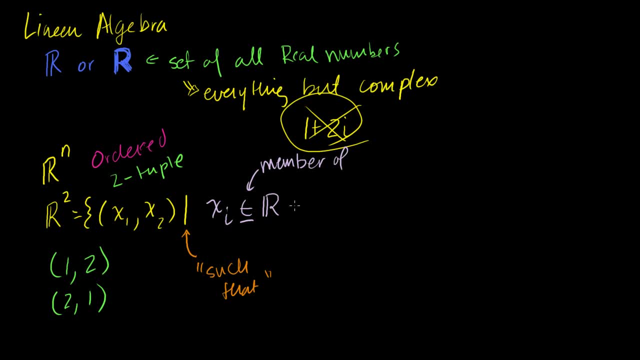 And I'll write 4.. 4. i is less than or equal to 2 and greater than or equal to 1.. And i is an integer. Now I could have written this a bunch of different ways. This is almost silly how much effort I'm taking to write this. 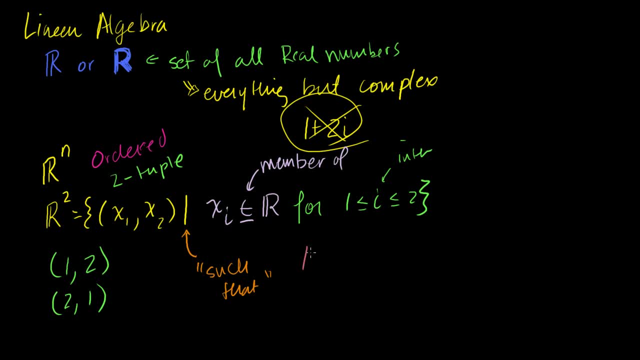 this way, But I could have written it like this too. I could have written: the r2 is equal to the set of all ordered tuples x1, x2. Such that x1 and x2 are a member of the reals. 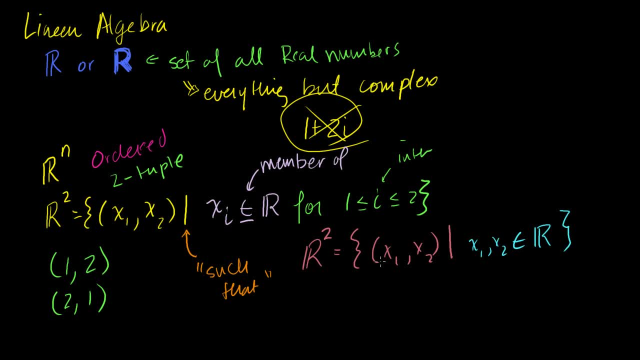 I could have written it that way. That would have been an easier way to write it. But either way, I think you get the idea. It's all of the combinations of two things. So I said in the beginning: this kind of is a squared. 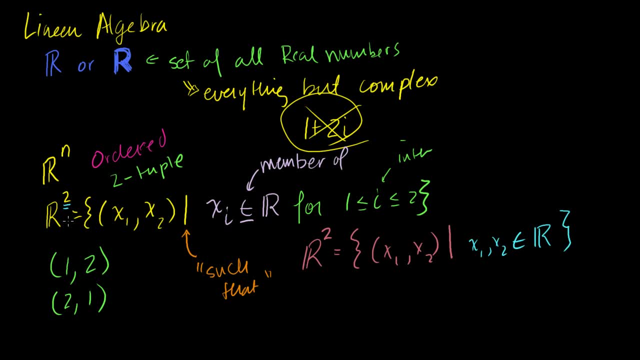 operator And why did they write it as a superscript there? And my gut sense is, if you think about it in this, you know You have kind of an infinite number of real numbers. I mean I won't go into things like accountability and 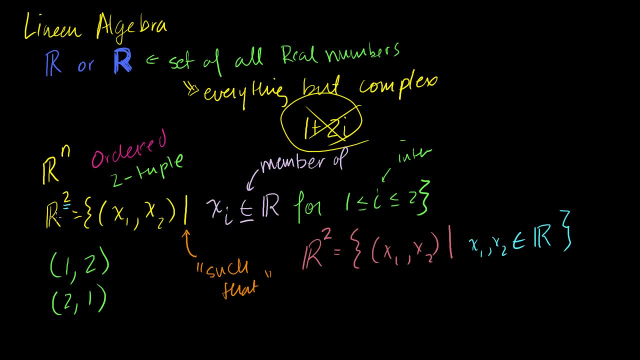 things like that. But you have a very large number of real numbers. But let's say that you only had n real numbers, right? Let's say that we weren't dealing with reals Just for sake of argument. let's say that you had, like. 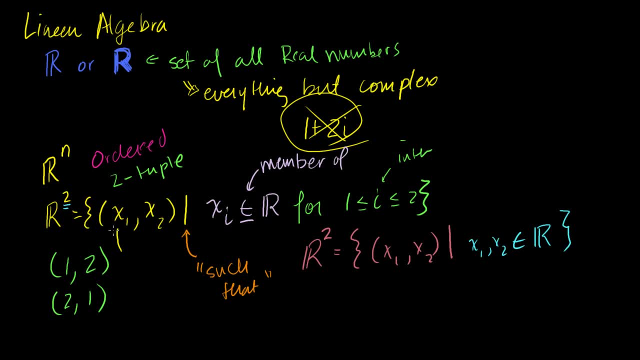 100 real numbers, right? So that means that there would have been 100 possibilities there, and then there's another 100 possibilities there. So now your set of all of the possibilities of two tuples. well, you'd have 100 times 100 possibilities. 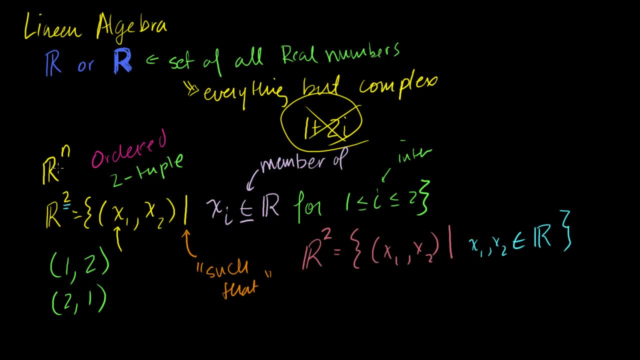 So you'd almost have the squared number of possibilities. So, however many possibilities you have for r, so you have that many squared possibilities for r2, which doesn't make a lot of sense because you have an infinite number of possibilities, but you have that many more. 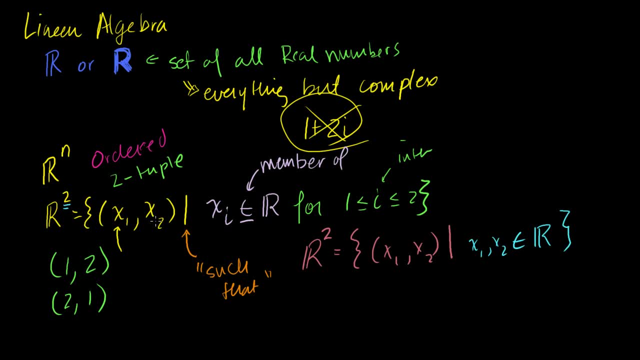 possibilities. You have an infinite number of possibilities here and an infinite number of possibilities here, So it's almost a greater infinity of potential possibilities. Now, what's r3?? r3 is just the same thing r3 is. if someone wrote r3, that means you're going to. 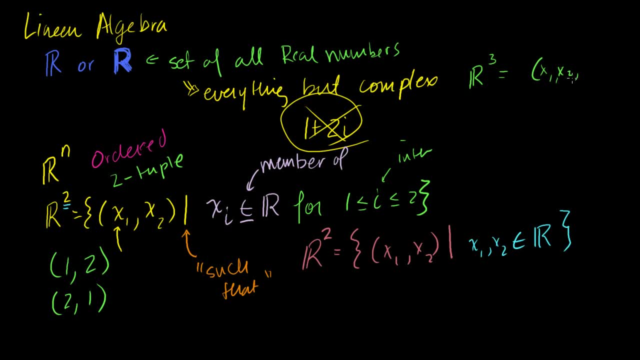 have three points or three numbers. I want to be careful not to just say points. We can graph these things and, for example, r2, points in r2 can normally be graphed on graph paper just in Cartesian coordinates. Points in r3 can be graphed in three dimensions. 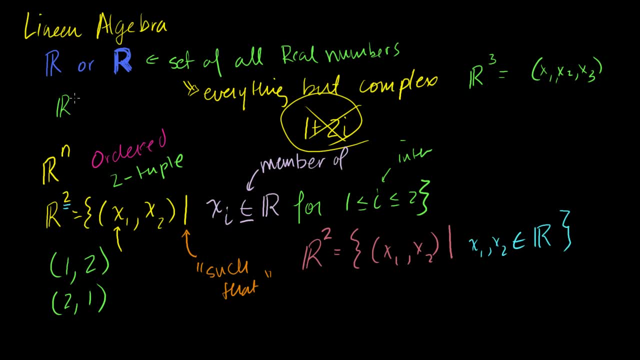 Points in just r, or we could just say r1,. you could just graph those on a number line. I could have a number line like that, and if I had to graph pi, that's 0, I'd just say: hey, right, there, that's. 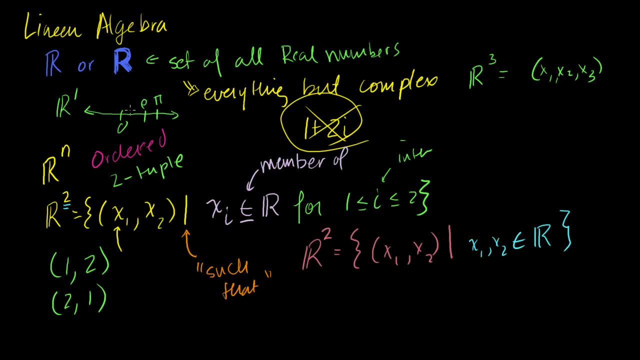 pi. and if I had to graph e, I'd say, hey, right there, that's e. and if I had to graph 1, I'd say, hey, that's 1.. So you could graph them, but I want to be careful that they. 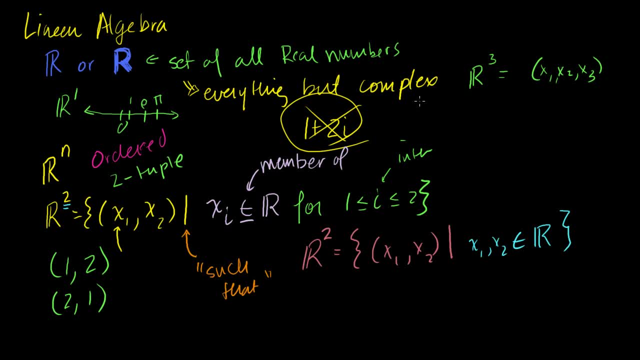 don't have to graph them, They don't have to correspond to actual physical points on a graph, But anyway, when you talk about r3, you're literally just talking about all the possibilities. You have an ordered set of three numbers where all three 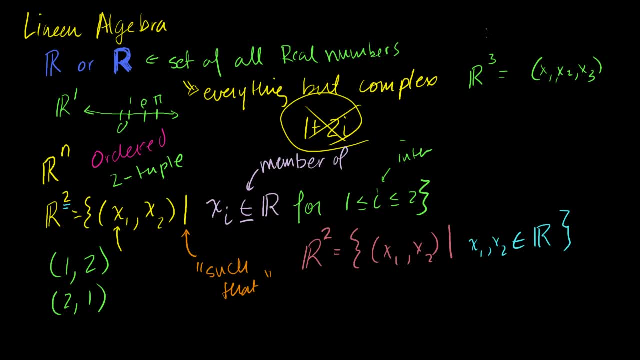 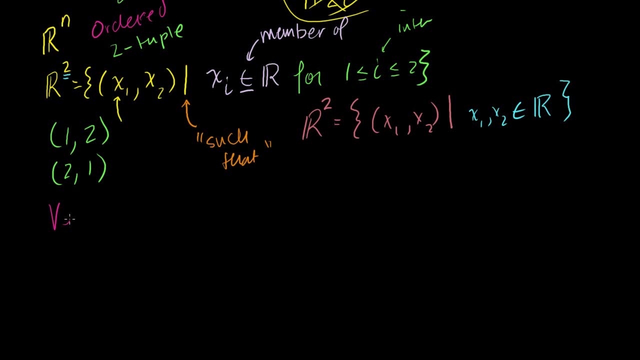 numbers are a member of the real numbers. That's all you're saying. Now I want to introduce you to another definition of a vector, Now a vector you've seen before. You've seen it in physics, where you said: oh it's. 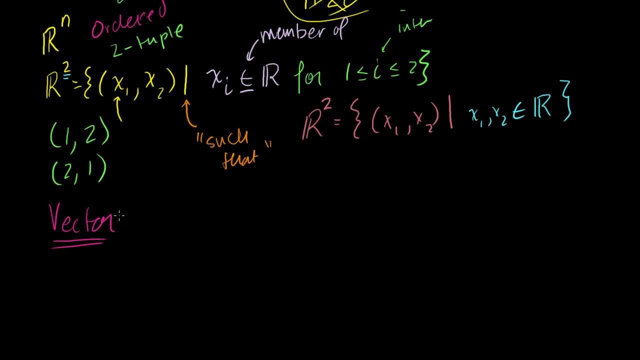 something that has a magnitude and a direction. You saw it in calculus and we plotted them and whatever not. But I'm going to be very formal and very abstract and very broad with the vector right now, Because I guess the beauty of linear algebra is that it. 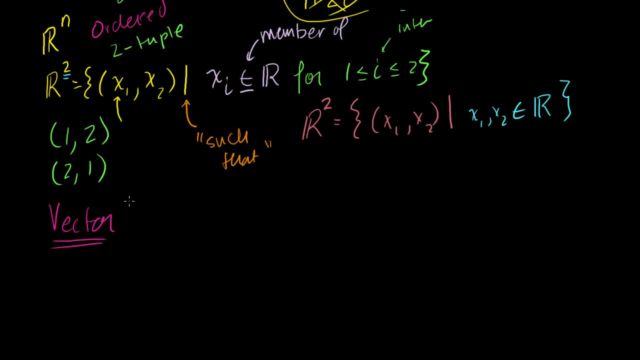 doesn't just apply to things like physics And it doesn't just apply. well, it does apply a lot to physics, but it doesn't just apply to that. In linear algebra you can apply it to anything. It doesn't have to apply to things that are just graphs. 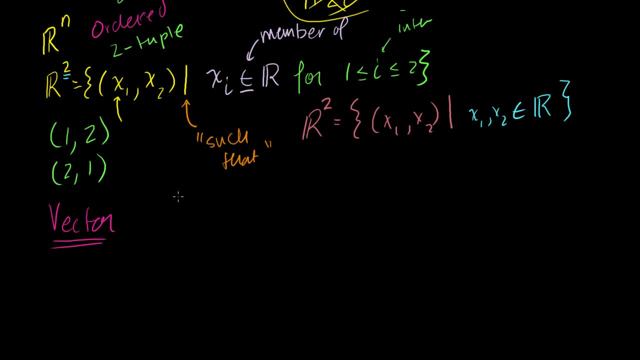 in three dimensions, And we'll talk more about that in the future, but that's why I'm trying to stay pretty abstract. So I'm going to define a vector in Rn, A vector to be in Rn. Actually, let me be careful. 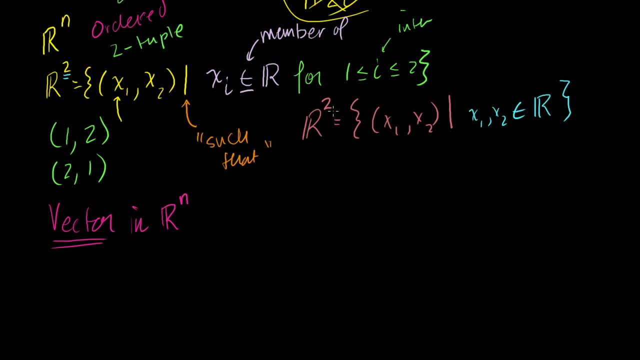 I haven't even defined what Rn is. I just defined R2 and R3. So let me define Rn. Rn is equal to the set of all n-tuples ordered n-tuples. So you have x1, x2, all the way over to xn. 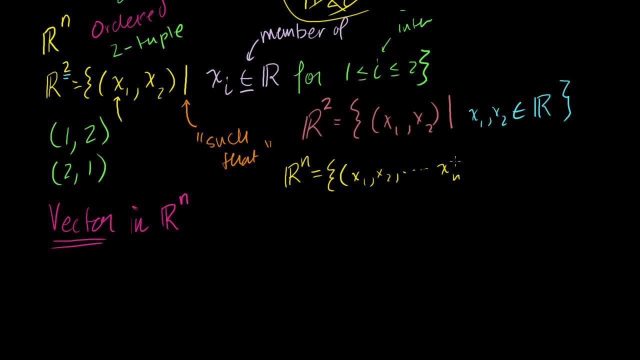 So you're going to have n things. So if this was 100, you would have 100 things here. So you have. this is an ordered Ordered n-tuple. This is an ordered n-tuple such that, for each xi, where 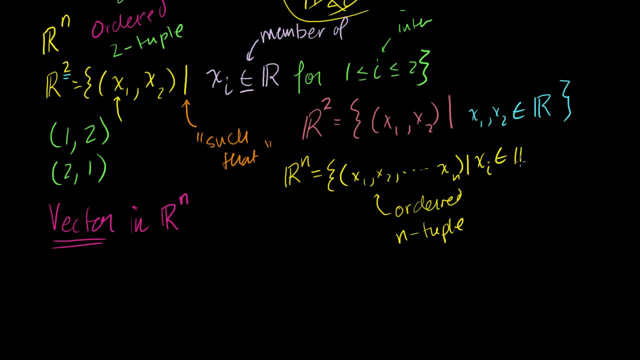 xi is one of these, is a member of the real. So each of these has to be a real number. And then I'll just say: for i is less than or equal to n, greater than or equal to 1.. So all that's saying is that for x, you know x1,, x2,, x3,. 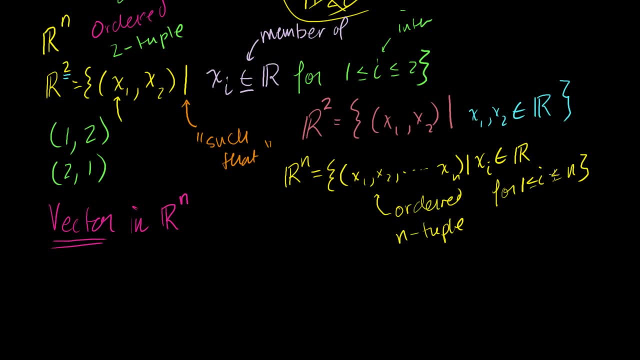 you know, x1 is a member of the reals, x2 is a member of the reals all the way up to xn is a member of the reals. Rn is the set of all of these possible ordered n-tuples or. 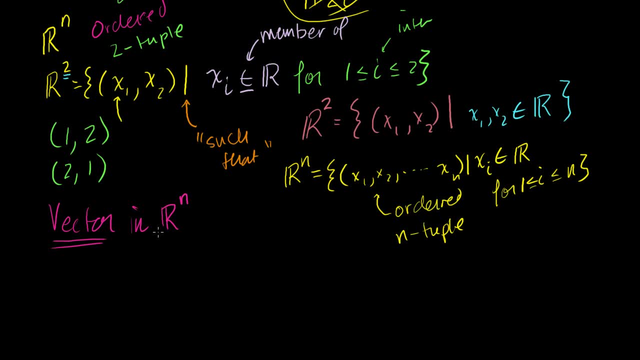 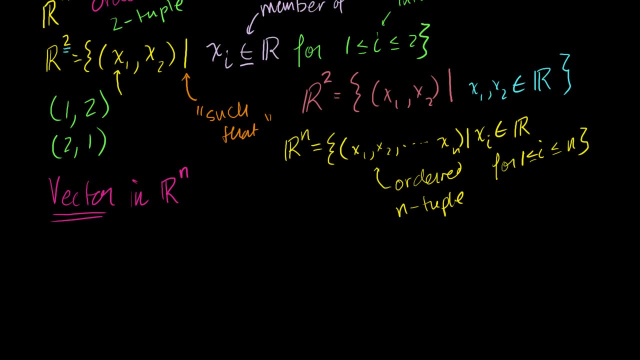 ordered sets of n numbers. So what is a vector? What is a vector in Rn? Well, a vector in Rn really is just a particular instance of one of these n-tuples. I'll just call it an ordered list, And you can represent a vector in a bunch of different ways. 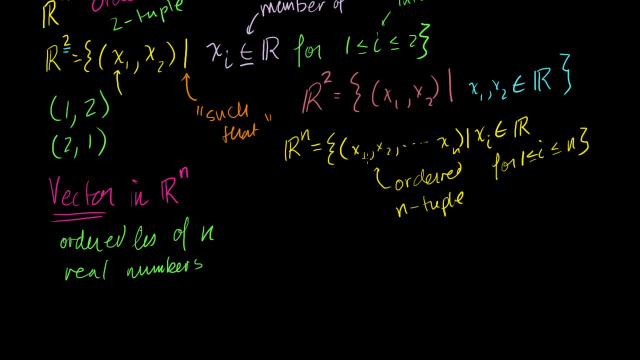 You could represent it like this. You could represent it like: well, let me do it in a bunch of different ways. You could, you know, a two-dimensional vector. you could represent like x1, x2, kind of like a coordinate. 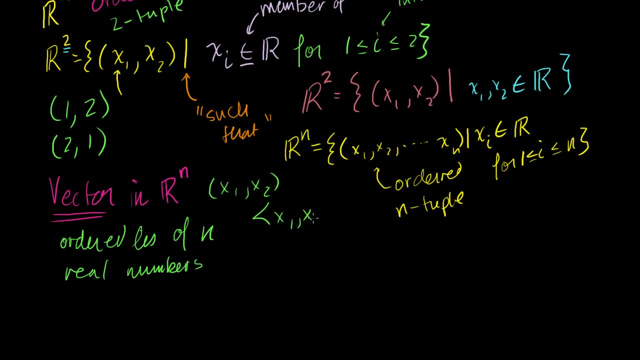 You could maybe represent it with brackets like that. This is just syntax. This is just different ways of representing the same information, the same idea And for most of what we talk about in linear algebra, we're going to represent them as essentially, these columns. 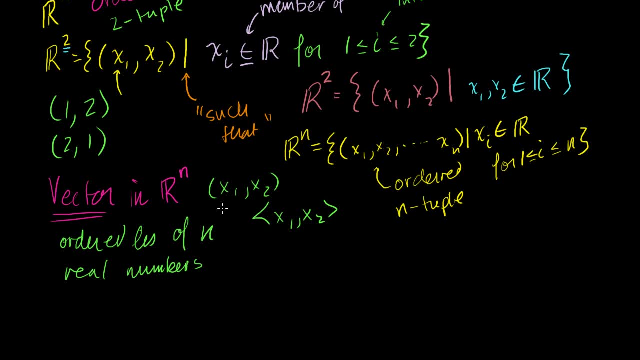 And in the very near future we'll represent them as rows as well. But I'm going to define my vector. A vector is an Rn is an ordered list of n real numbers, and I'll define it, And this is an example. 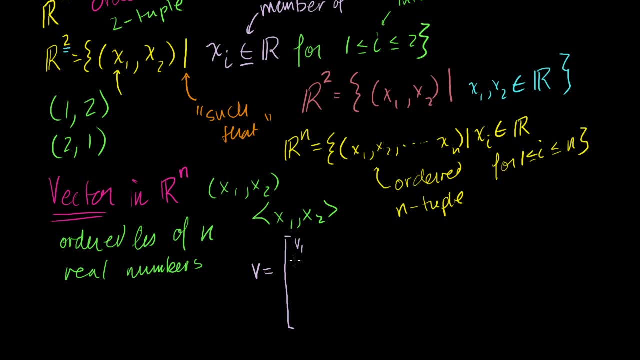 So it would be v1,, v2, all the way to vn, where each of these were. Each of these is a member of the real numbers And, just to make sure you kind of understand the notation or the terminology, each of these is called a component of our 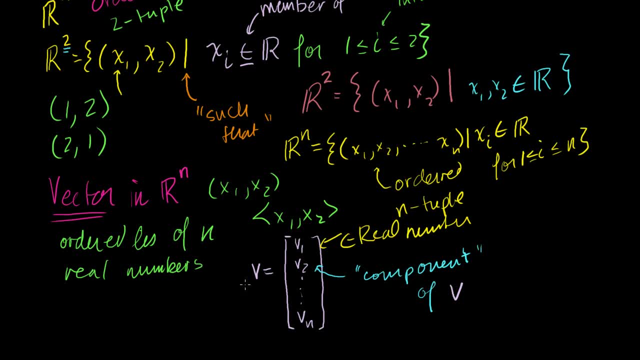 vector And actually I want to be very careful here, Because when we write vectors you want to make sure you have a nice bold v. I won't make all my v's. I won't make all my v's in the future that bold. 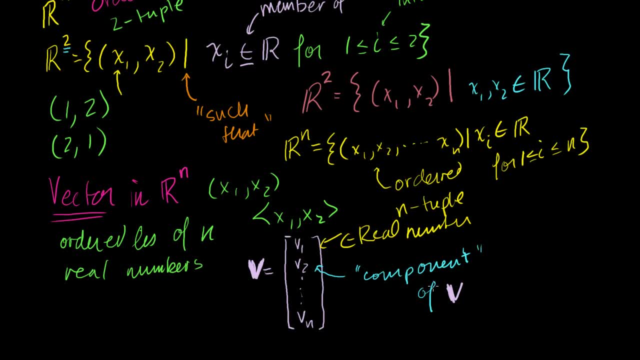 But that's how, when you're reading a math book, they differentiate between just a vector and just a regular quantity, right? These regular quantities are just written with a non-bolded, while the vectors are bolded. Now I'm going to define two definitions for vectors. 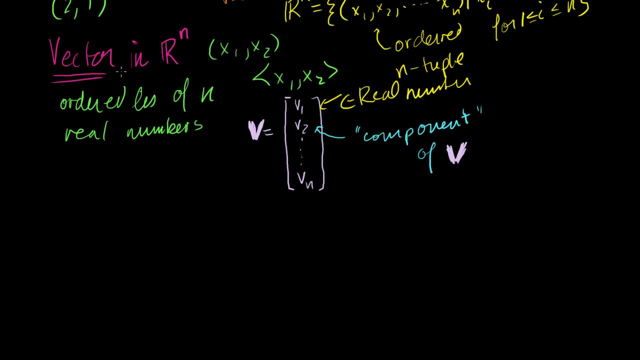 Two operations for vectors in Rn I'm going to define addition And these are definitions. I could define them in r: poverty Aren't you Any arma arbitrary way, but these I think you'll find to be somewhat natural. So these are definitions. 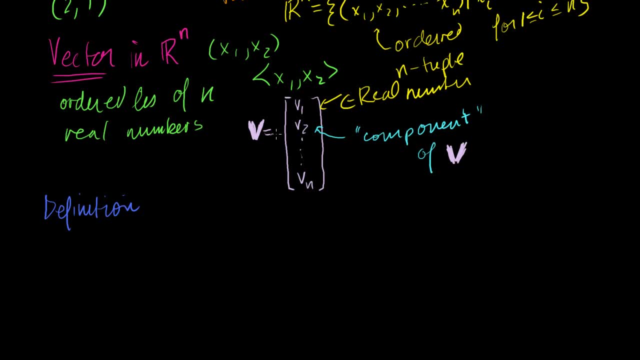 These are just kind of human abstract constructs that end up becoming very useful. So they said: hey, let's make some definitions, Let's define addition. So if I have some vector, let me write it as a lowercase a, but it's a really bolded lowercase a. 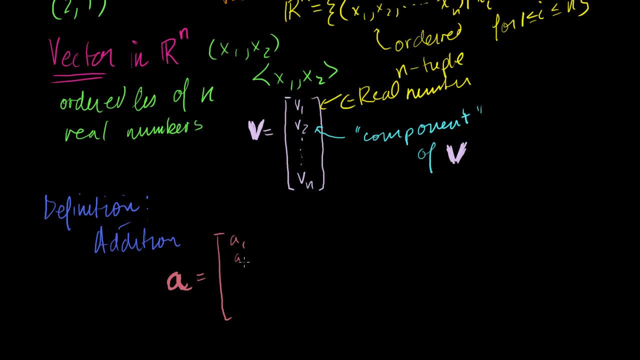 And then that is equal to a1,, a2, that's all of its components, all the way to an, And I want to add that. and then I have vector b and I'm going to make that a really bolded b. right, there is equal. 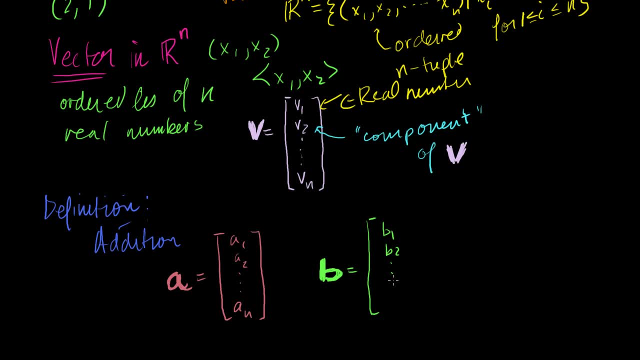 to b1, b2, all the way to bn. I'm going to define addition of these two vectors to be just the sum of each of their components. a bolded a, a plus bolded b is equal to a new vector where you just add. 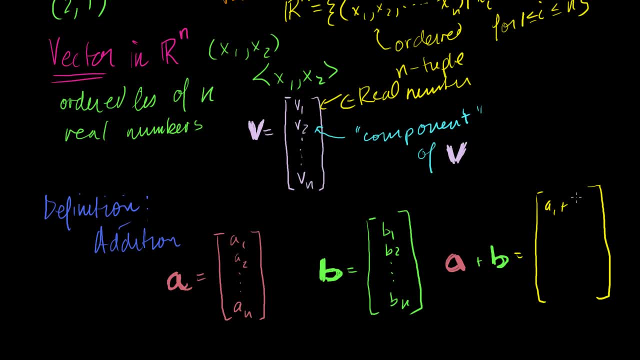 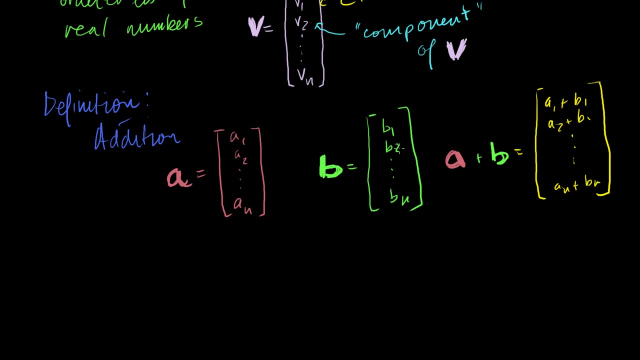 each of their components. It's going to be a1 plus b1, is going to create this new component, a2 plus b2, all the way down to an plus bn- And if you found this somewhat confusing, I'm almost going through pains- to write something very simple in very 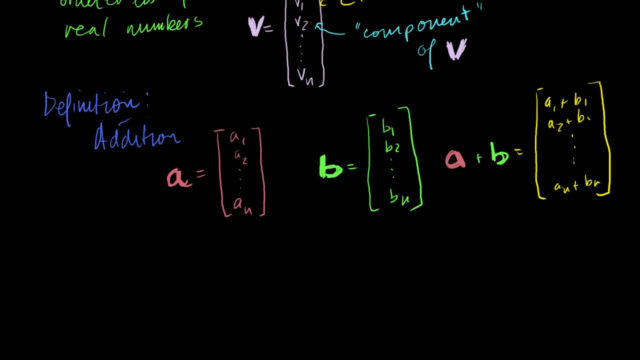 confusing terms. If I have two vectors in R2, let's say I have the vector 2 minus 1, and I want to add that to the vector 3, I have 2, I literally just add each of the corresponding components. 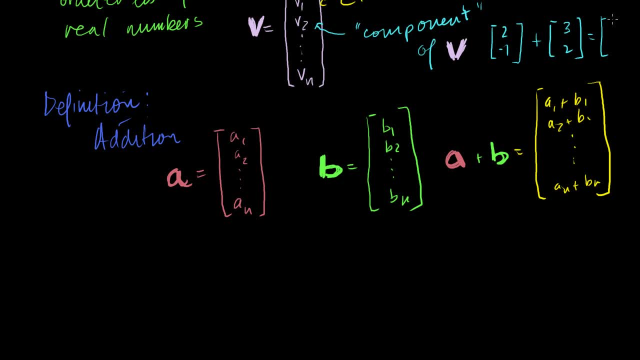 So I add the first components to each other. So 2 plus 3 is equal to 5, minus 1 plus 2 is equal to 1.. That's all my definition. That's what a vector addition is for my vectors in real. 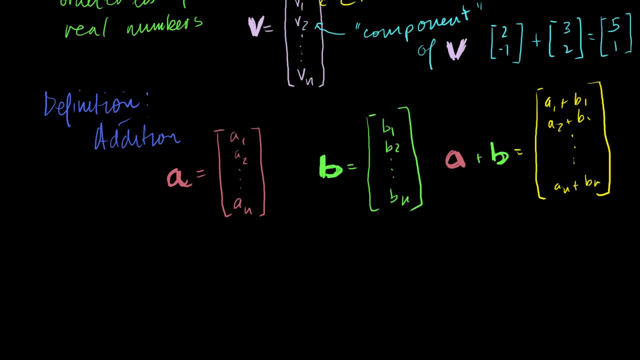 numbers. And now the next thing I'm going to define is the idea of a scalar multiple. So scalar multiple- You might remember from physics class a scalar- is just a regular number. If you're multiplying something by a scalar, you're just scaling it up. 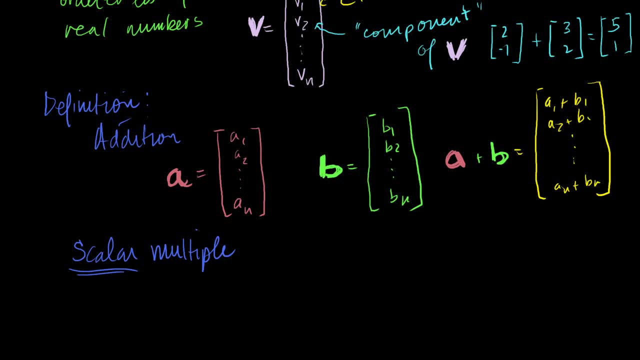 Maybe I shouldn't use the same word in the definition, But I'm going to define it as, let me say, c is a scalar, So let's say I have some. I notice I didn't bold the c, So c times my vector a. and here I'm going to take pains. 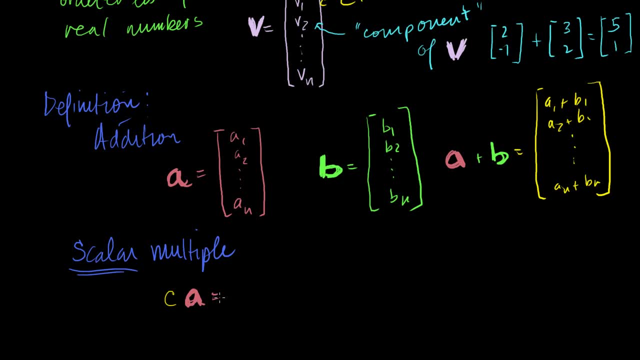 to bold it up times, my vector a is going to be equal to all of my components of vector a multiplied by each, multiplied by c. So a1, a2, all the way to an, and they're each going to be multiplied by c. 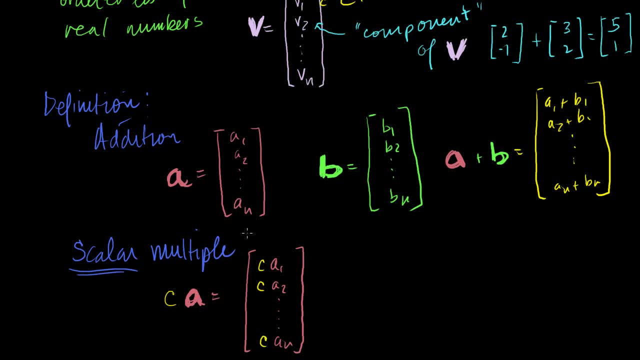 So that's all I define Every term. Every term is going to be multiplied by c And just to give you an example like that, if I wrote minus 3 times some vector, I'll just draw the vector here. Let me draw a vector in R3.. 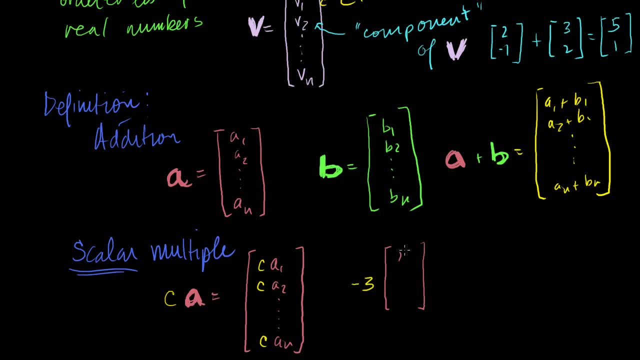 So let's say the first term is pi, the second term is minus 2, and then the third term is 0. Then this is just going to be equal to. This is just going to be equal to A new vector in R3, or you can kind of view it as a.